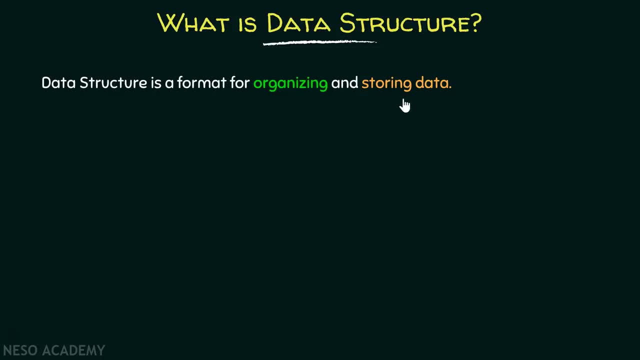 It is a format in which you can organize the data. Also, you can store the data Also. each data structure is designed to organize data to suit a specific purpose. For example, an array is a data structure which you can visualize as follows: 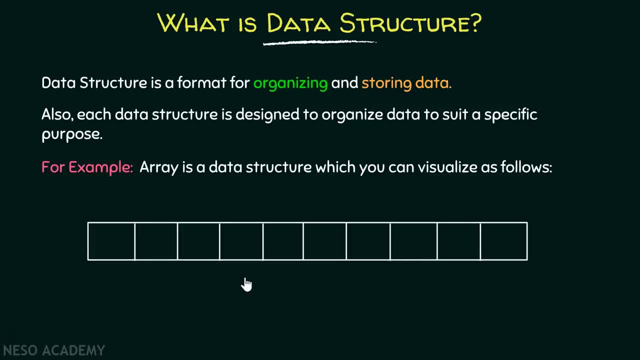 This is the way you can visualize an array. It's a large chunk of memory divided into smaller blocks of memory, And each block is capable of storing a data value of some type. This is the way you can visualize an array. It's a data structure. 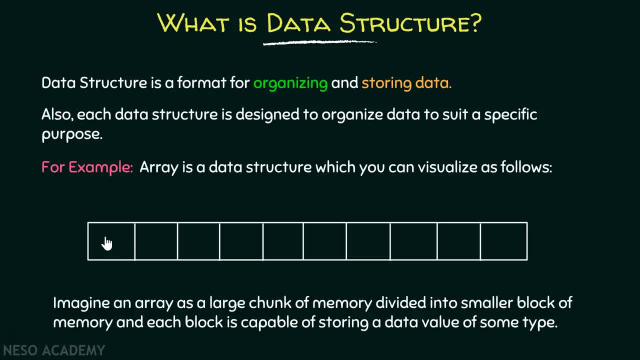 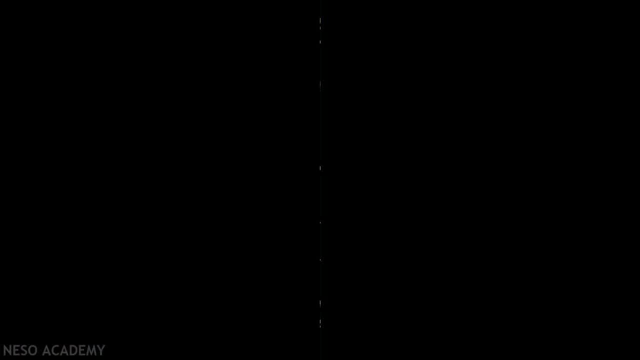 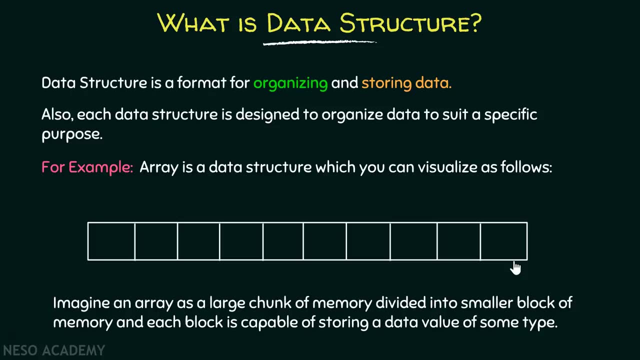 Because here you are storing the data as well, as all the data is organized in a sequential manner, right? That is why an array is a data structure. In each block you can store some data of some type, And all of them are organized in a sequential manner. 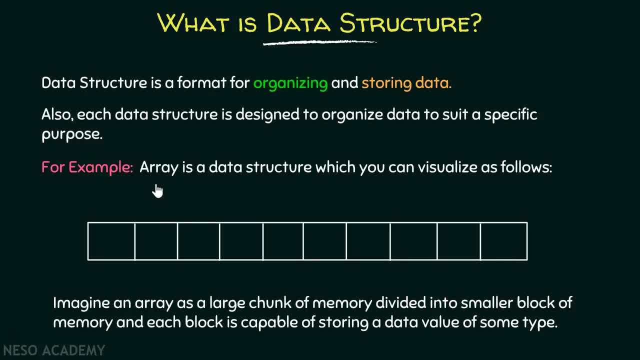 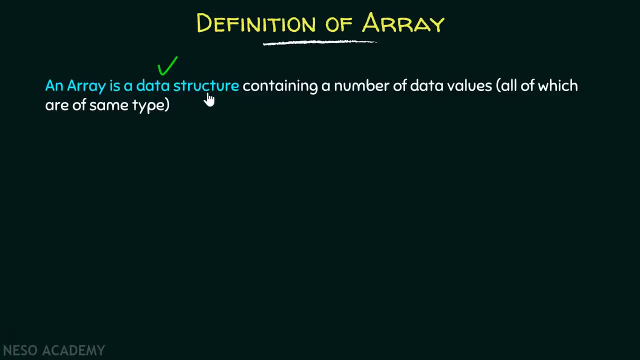 So we can understand that an array is simply a data structure, right? So the first part of this definition is very clear: that an array is a data structure. Let's come to the next part. It contains a number of data values. 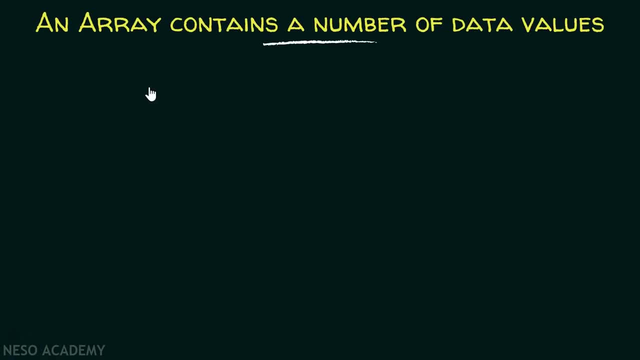 What does it really mean? This array consists of ten data values. You can see, this array consists of ten data values, all of which are integers, and each value is stored in a separate block of memory. Right, So we can say that an array contains: 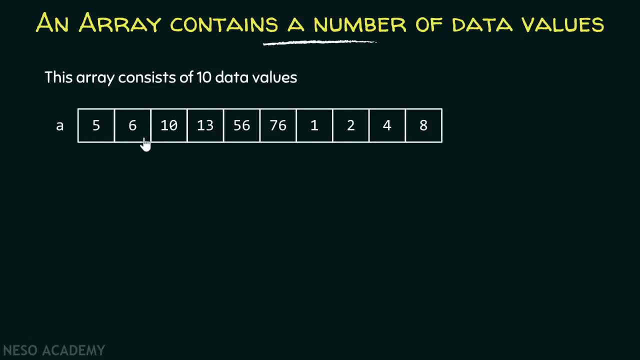 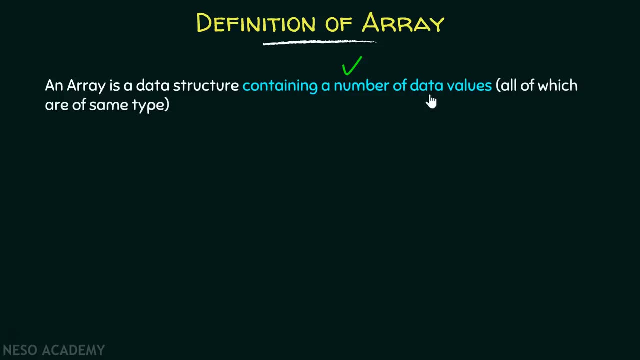 a number of data values. This array contains ten data values. Similarly, this array contains five data values, And again all of which are of integer type. So the second part of the definition is also clear: that an array consists of number of data values. 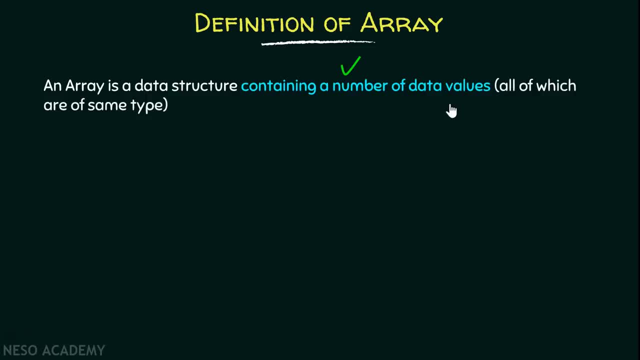 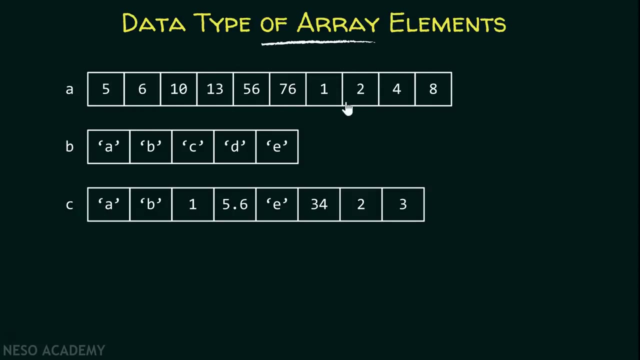 Right, Let's come to the third part of this definition, All of which are of same type. Let's try to understand this third part as well: Data type of array elements. This array consists of all integer values. Right, And this array consists of all characters. 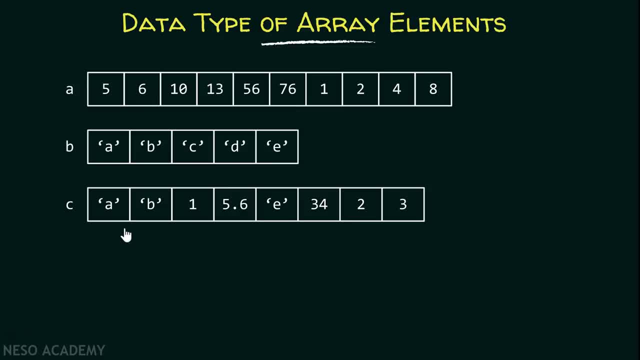 But what about this array? This array consists of characters, integers, floats, But the definition says that all elements must be of same type. So I can say that this is correct, this is correct, but this is not correct, Because the type of all these elements